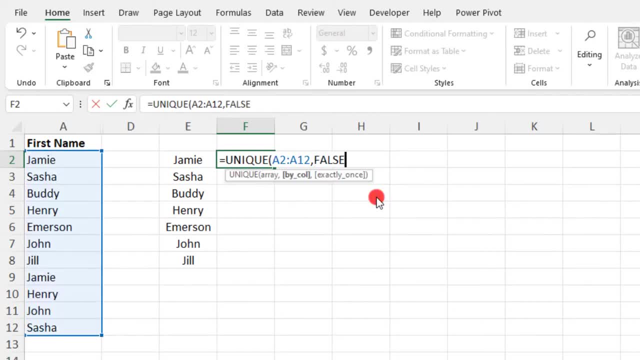 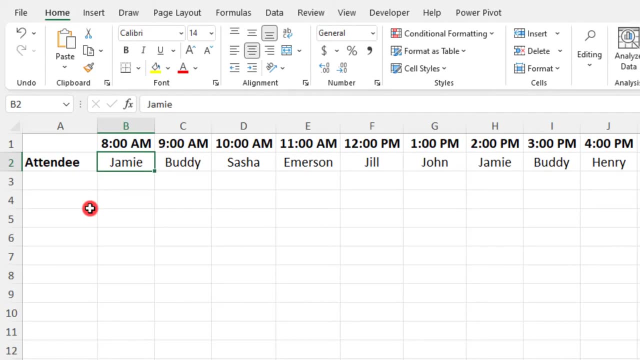 But typing false here to return unique rows will give us the same result. Now, sometimes you may need to use the unique function along columns, or in this case, where the list is in a row, but each item that we're going through is in a row. 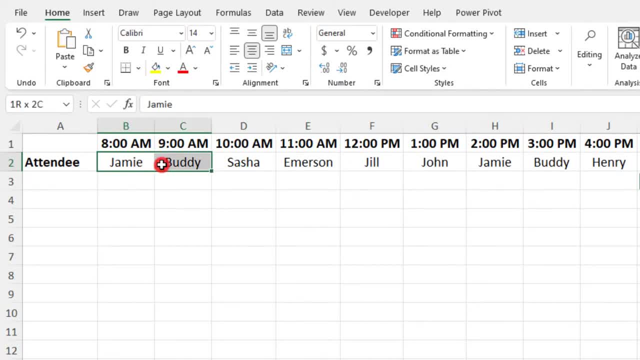 So what we're going to apply the unique function to is in a different column, so column B, C, D, E, etc. So in this case, if we wanted to get the unique values across these attendee names, we would type: equals unique. select the names. 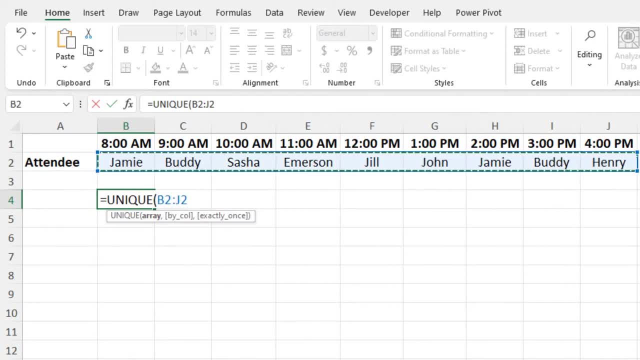 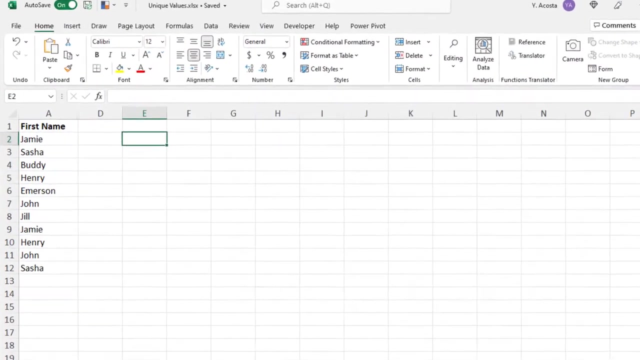 Again, don't forget to omit from your data any headers, And this time we want to type true, because we're looking across the columns And now we can close our parentheses. You can also use the unique function to generate a list that omits anything that is listed more than once in your selected data. 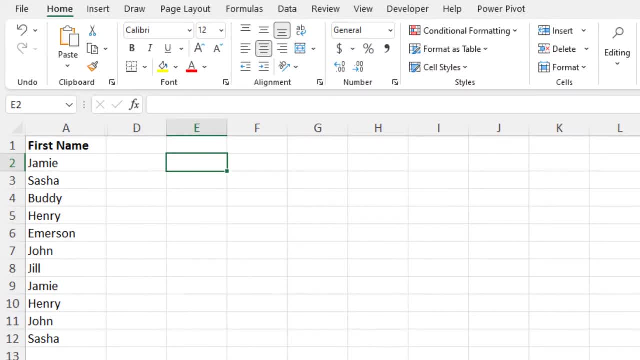 So, for example, in this list of first names only Buddy Emerson and Jill appear. once All the other names are repeated, You can also use the unique function to return only Buddy Emerson and Jill. So to do this: type equals unique. select your data. 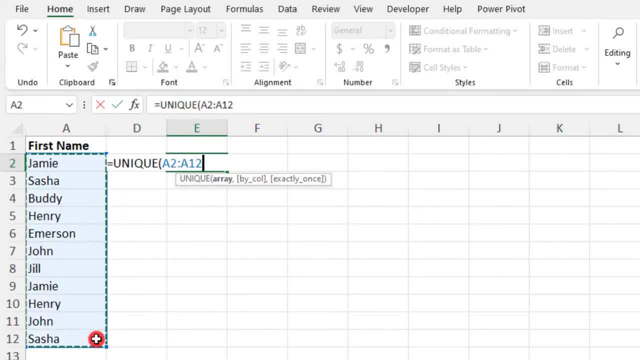 and because our items are listed in the default layout, we can either type false for the second argument or type two commas and skip it altogether. And then the third argument: you can select any items that appear in the default layout that appear exactly once, which is what we want. 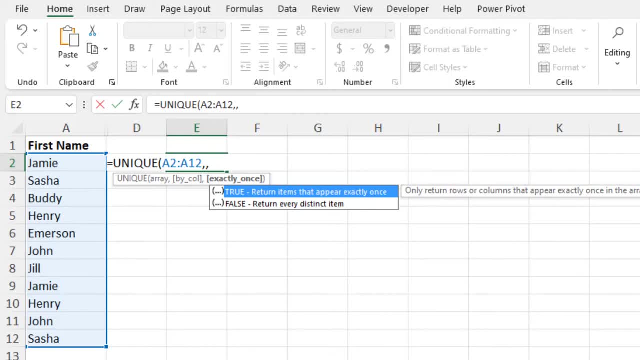 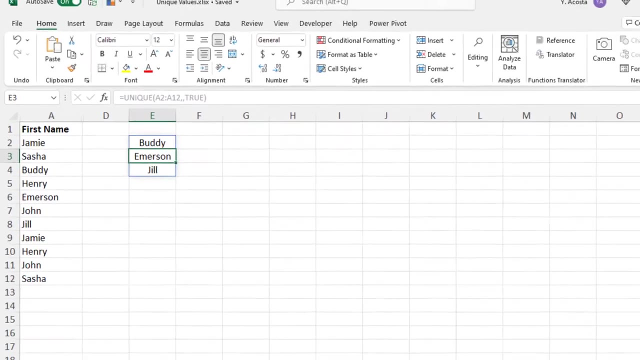 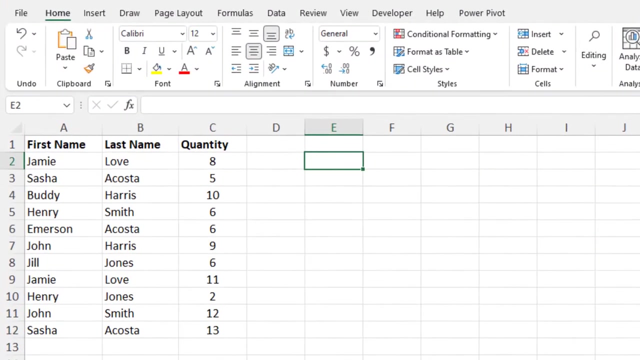 or the default, which is return every distinct item, But because we only want items that appear exactly once, we'll type true, close our parentheses and now we have a list that just shows Buddy, Emerson and Jill. You can also use the unique function to find unique values that span multiple adjacent rows or columns.